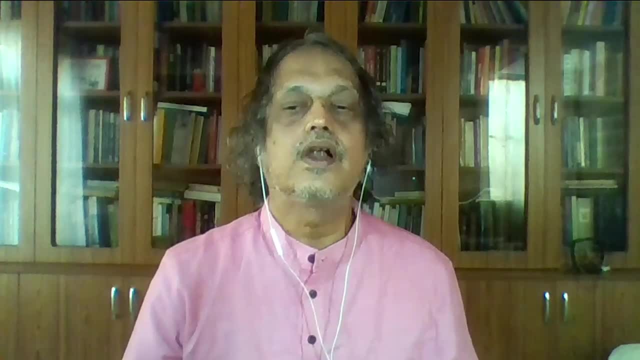 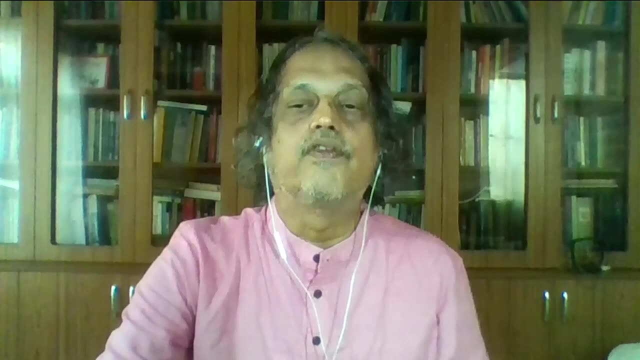 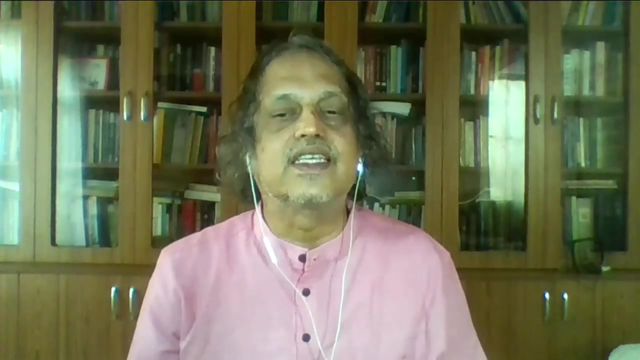 quantity. In this world of excess, the only thing that we don't seem to have is time. How do we respond to this point of excess? in everything that we do, We have also led to a great amount of this pandemic of excess in inequalities in society. The pandemic has 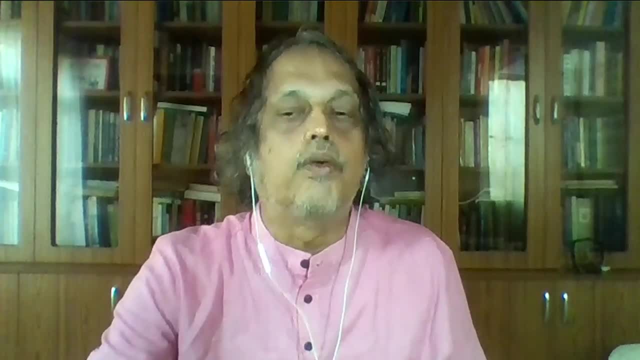 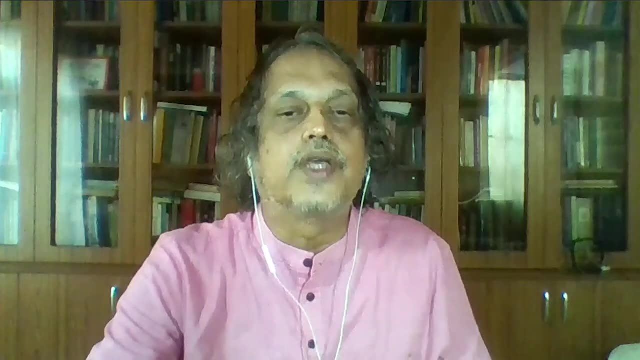 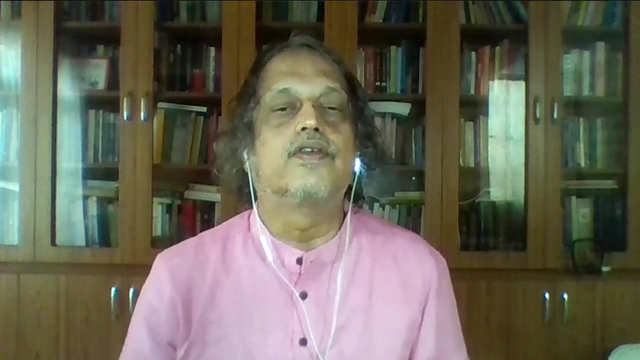 pushed millions of people back into poverty. This kind of a problem has also become an extremely important problem in education. There are, if you look at education, systems around the country. we have also caught up in the world of excess of disciplines and of information, And in a world full of. 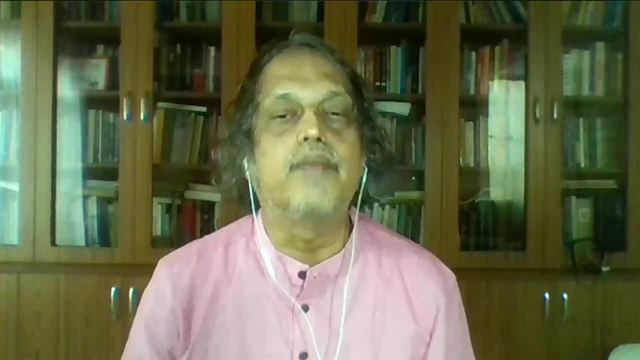 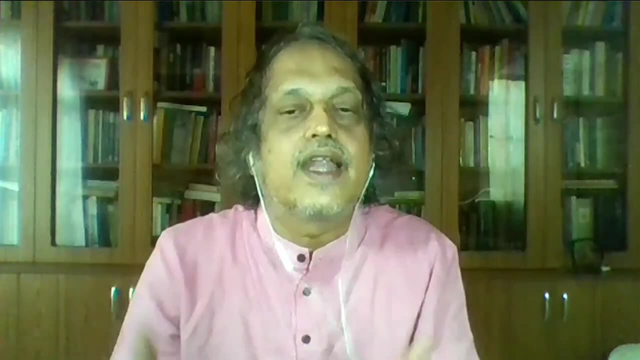 excess of disciplines of information, education has to take on a different meaning. If historically, the meaning of education was to accumulate and understand the content, today it no longer can do that. Maybe a few students in a class can do well under these circumstances. But 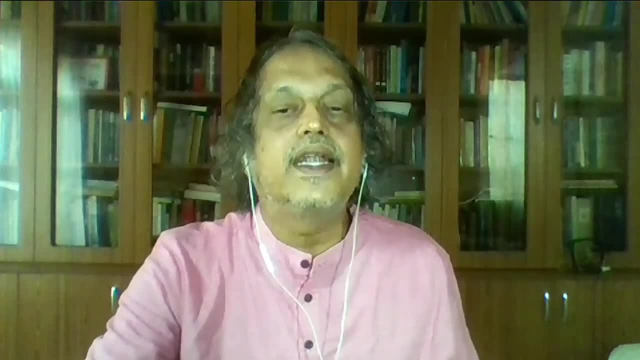 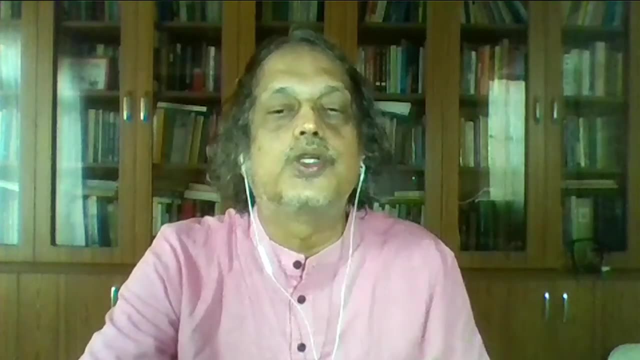 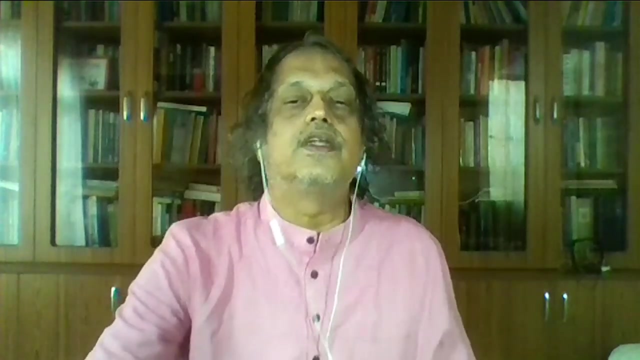 the value of education is its democratic nature, and it has to be inclusive more than anything else. Because what has happened in this pandemic world to education? Education, too, suffers from the problem of excess. There is an excess of disciplines. A listing of the number of disciplines, for example. 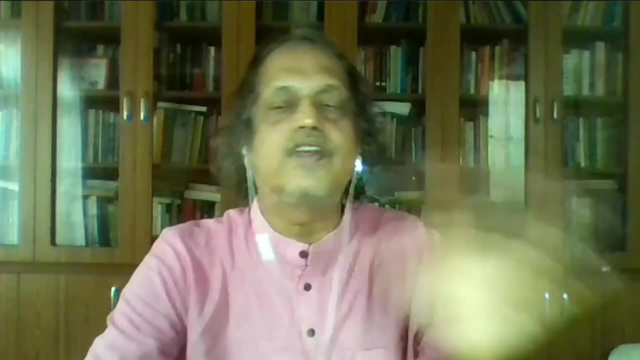 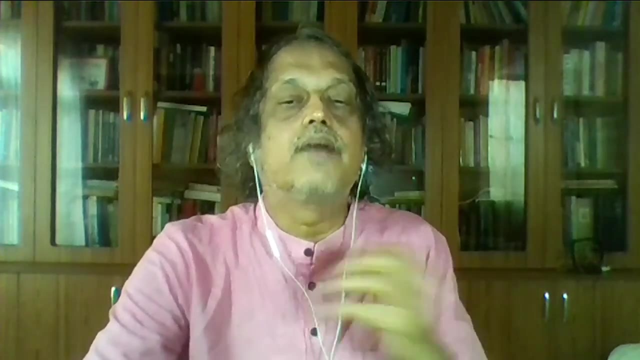 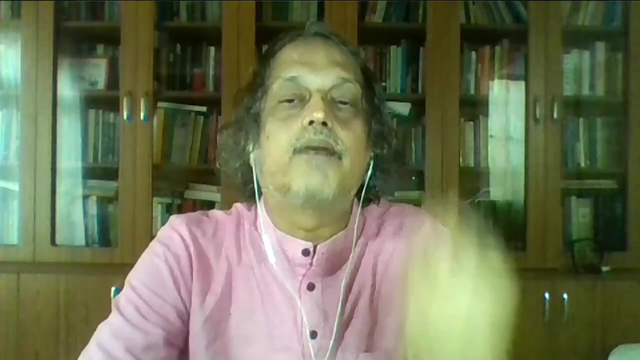 in biology alone runs into hundreds, many of which have separate departments and programs. So also in every other discipline belonging to science, content of knowledge has become unmanageably large. Even research publications have become excessive. Today, as many of you might know, we publish nearly two to three thousand articles a day. So there is a huge 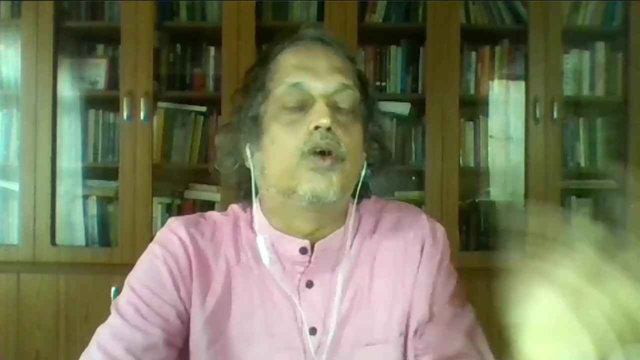 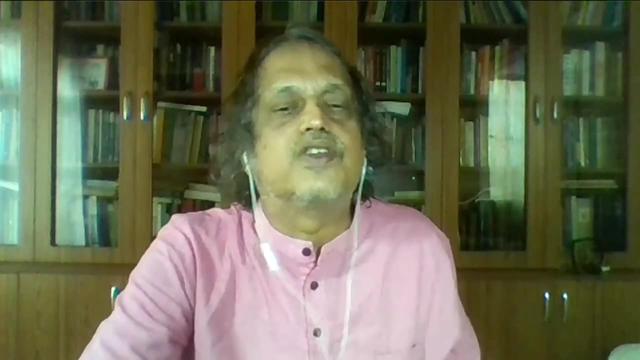 million two and a half to three million papers a year, which works out around seven to eight thousand papers a day which are published in science. And how are we supposed to read through this massive production? Today, scientists need curators and librarians to help them read, and 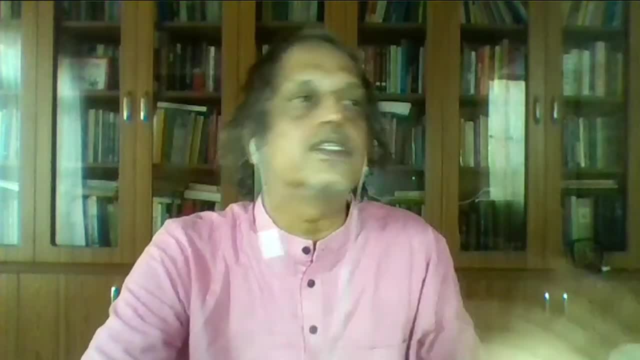 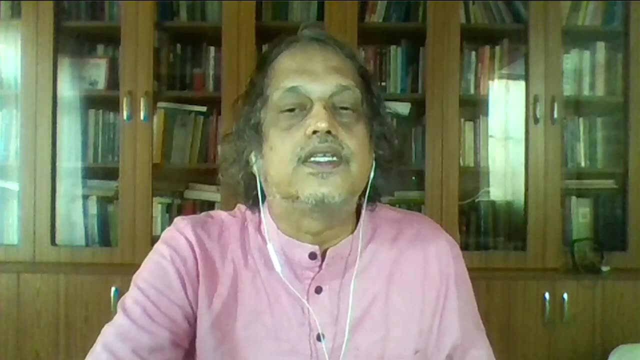 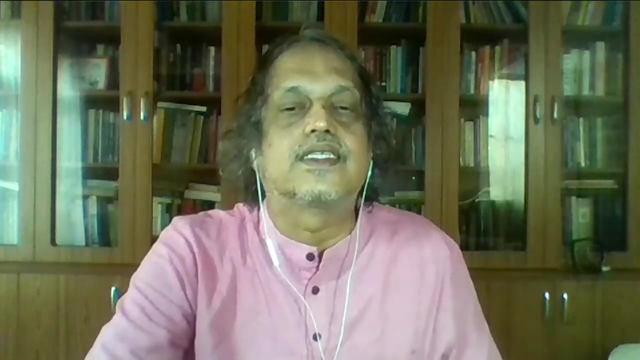 manage the enormous content. School teachers are in no better situation, as they do have to depend upon a huge amount of material from which to choose what to teach. So how can we get out of this mess that we are in today due to this large cultural and educational excess? I believe that 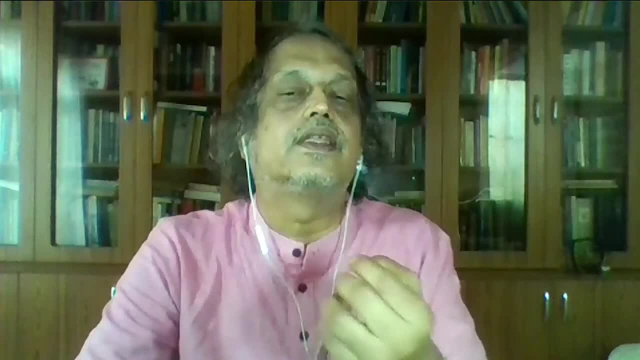 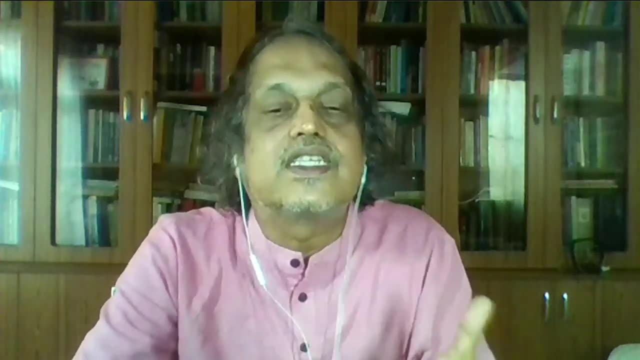 one of the best ways to accomplish this is to teach philosophical thinking to children right from school. There's a growing movement to bring philosophy to children in the West, and some common justifications for teaching philosophy to children include the following: You know they say that 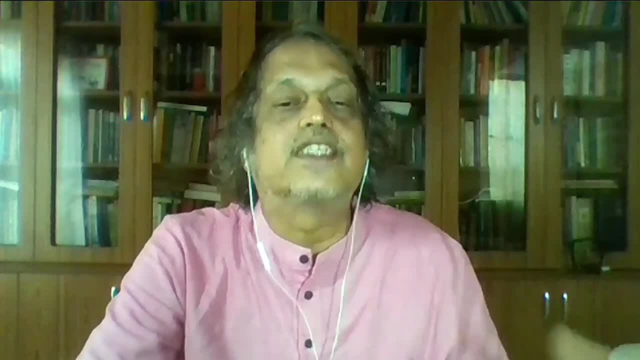 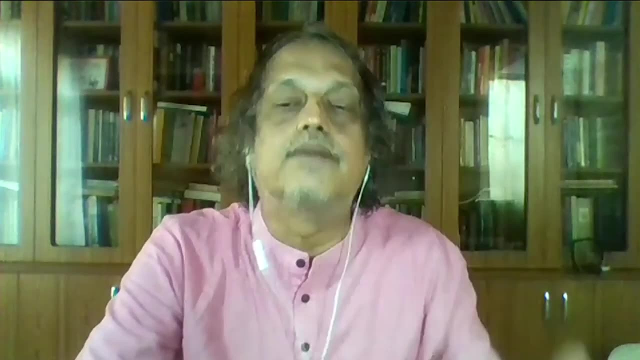 kids ask questions. naturally, Philosophy deals with big questions of life. It can teach you ideas of right and wrong, And especially in today's world where everybody is worried about ethics, that becomes essential. And it's essential to also teach critical thinking and logic and so on. So these are good reasons to teach philosophy. 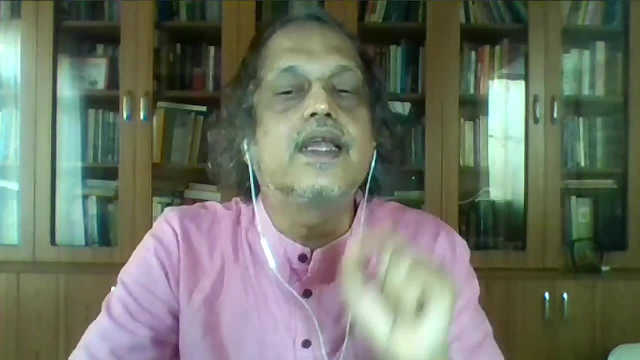 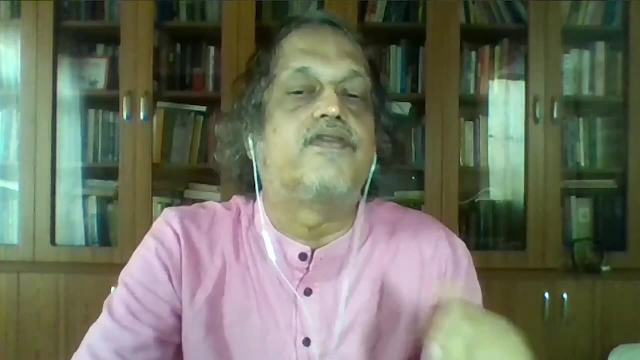 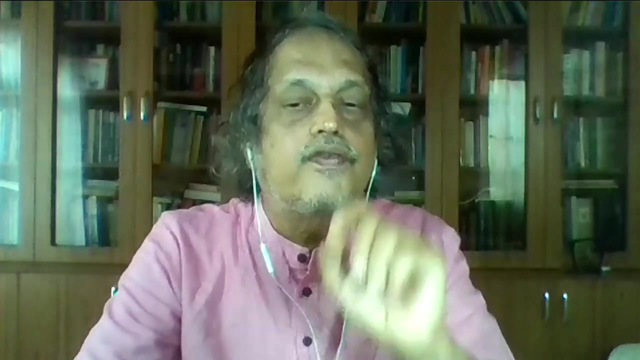 But we should remember that, along with these skills, there's another important task of philosophy, which is that it develops the capacity for critical reflection, self-reflection and to be open in principle to completely different perspectives. So the strength of philosophy is its ability to unify and synthesize. 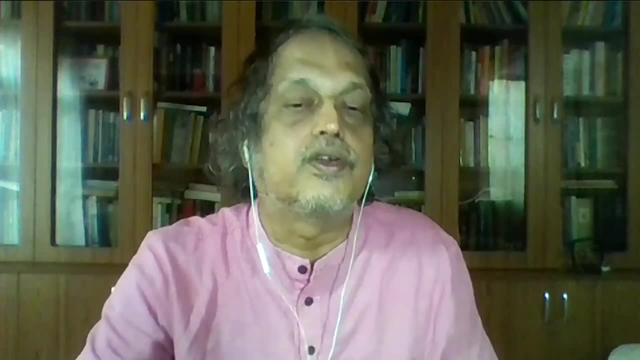 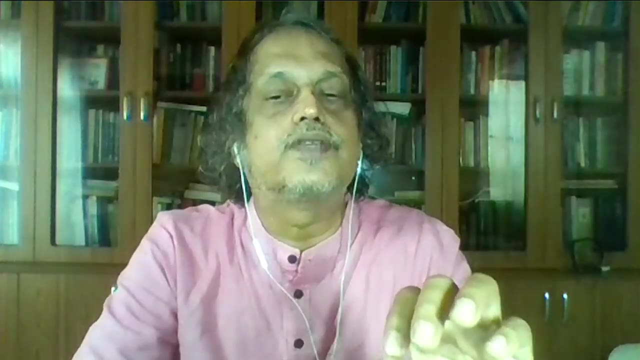 What seemed to be great differences, and this is much needed today. So in the case of India and more generally in Asia and Africa, it's absolutely necessary to teach philosophy to children, because we are- most of these countries are- caught in the middle of global education wars. Our paradigms of 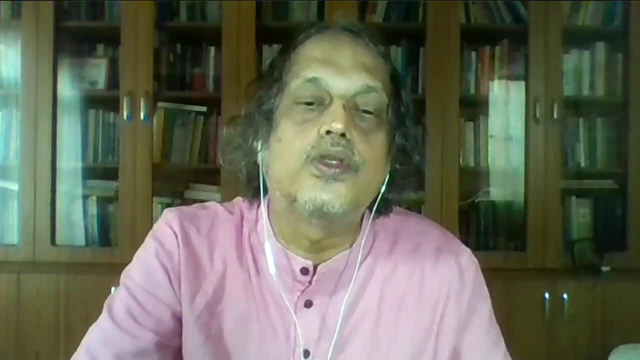 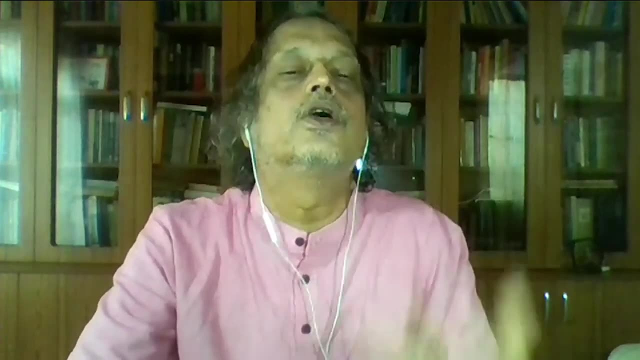 education are coming from elsewhere, under different kinds of forces, And, as some would say, there is a need to decolonize education in all these places. And why would we do that? Because you want to make education more inclusive. You want to make education more inclusive. You want to make education more. 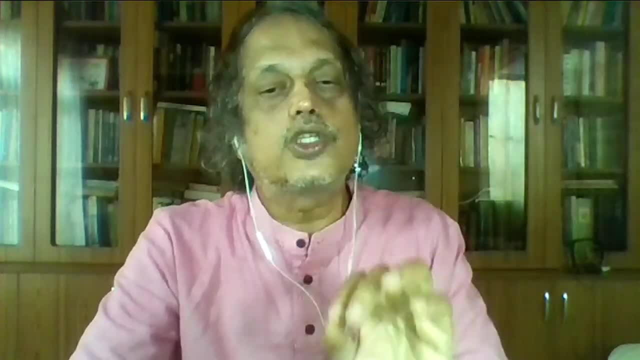 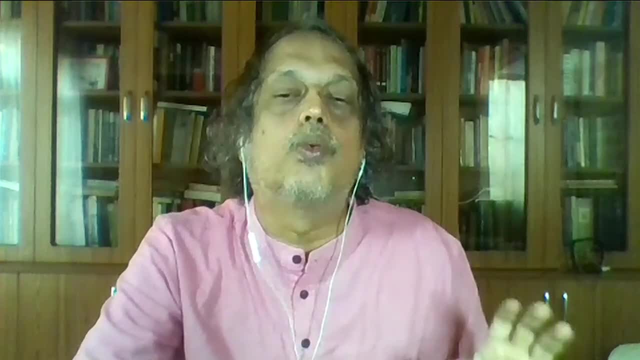 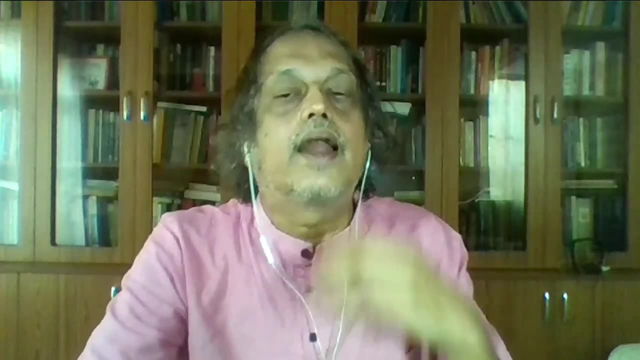 approach of teaching philosophy to children. This is based on the workshops on philosophy that I've conducted for children with the help of my students and members of our organization, Barefoot Philosophers. Our attempts to teach philosophy was primarily as a way of thinking about perception. 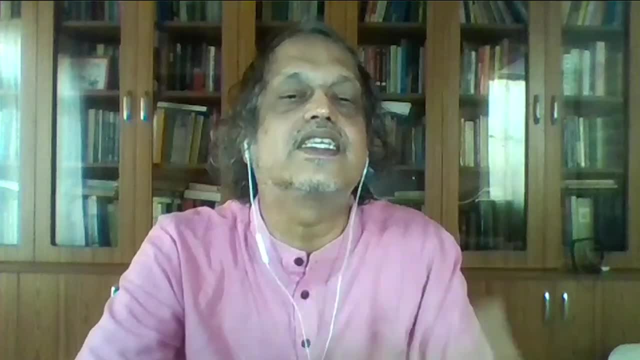 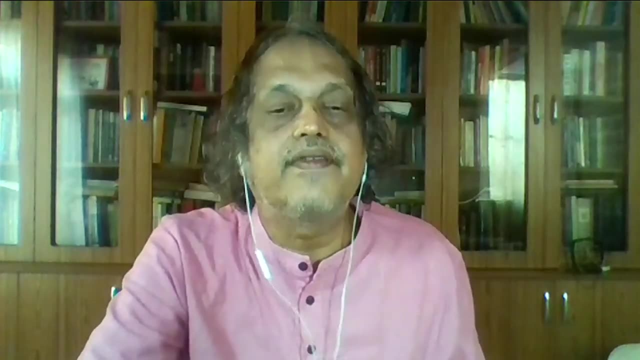 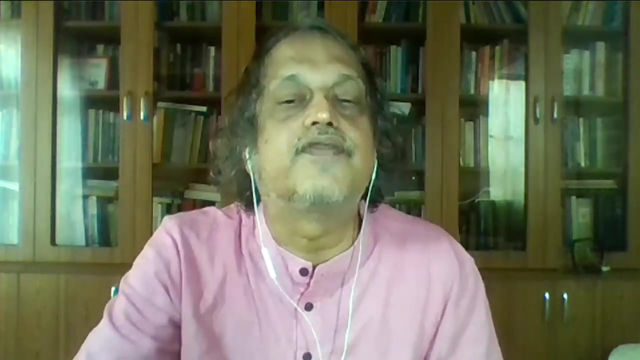 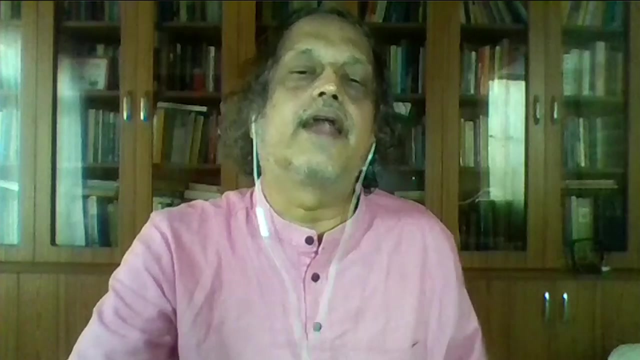 thinking, reading, writing- you know the basic things, the basic skills that you need to work in any discipline. It is first meant for students in class five to seven, because I thought that is the domain we have to focus, But we found that this model was useful across different grades and ages. These sets of workshops also led me to write a book called Philosophy for Children- Thinking, Reading, Writing- from which some of the examples I give below are taken. 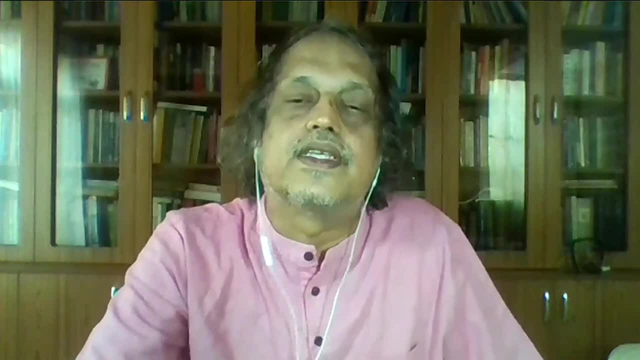 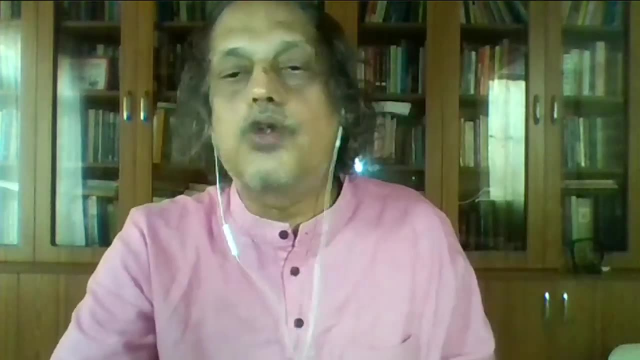 When I first announced workshops on philosophy for children, it was met with skepticism. You know, I was told that children don't want to learn philosophy and they're already learning too much. And, more importantly, I was told repeatedly that parents do not want to send them to. 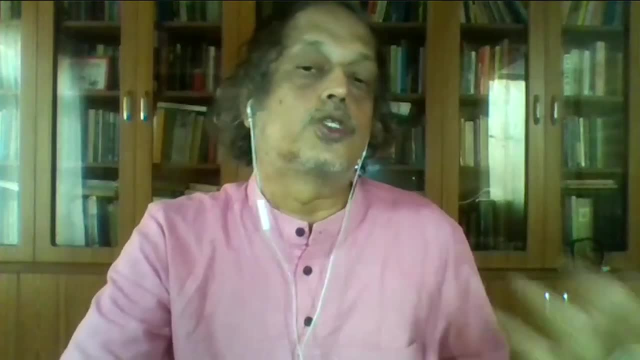 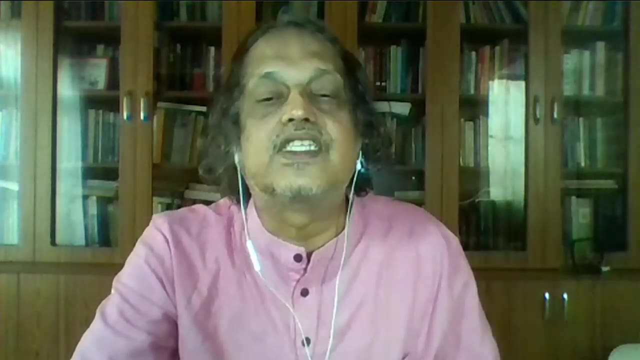 such workshops. But the first workshop got so many responses that I couldn't accommodate many of the students. so in response I did a series of workshops in different places, both urban and rural and, more important and very important in the context of India and in. 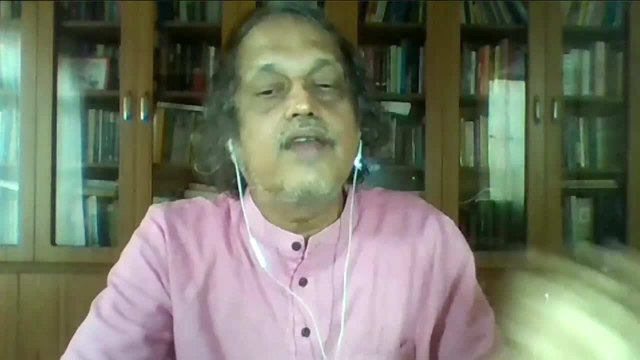 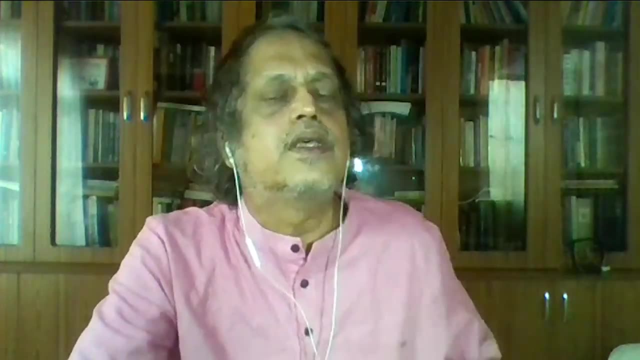 languages other than English. So everywhere we found real deep interests among both children and parents in learning philosophy. And this was a big lesson for me, because many of the the parents and felt that if the children had had philosophy teaching in their schools, maybe they 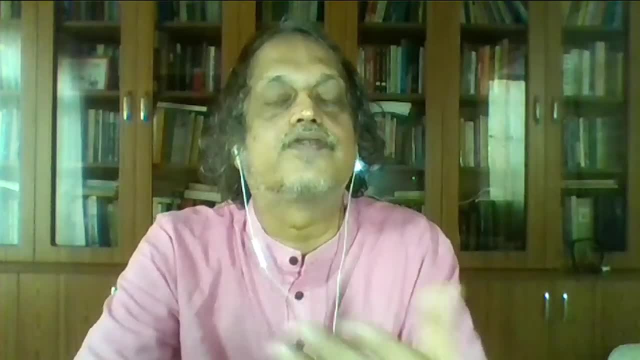 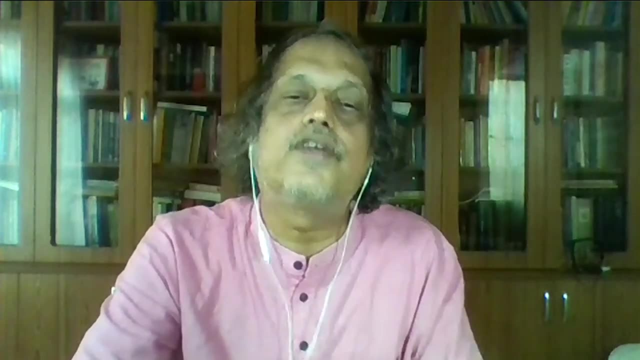 would do better in their other subjects, and that was a great sense of support to what we were doing. it was always, it's, it is always a challenge deciding what to teach under the name of philosophy, you know, whether it's for young students or my post-graduate and PhD students, do we teach some? 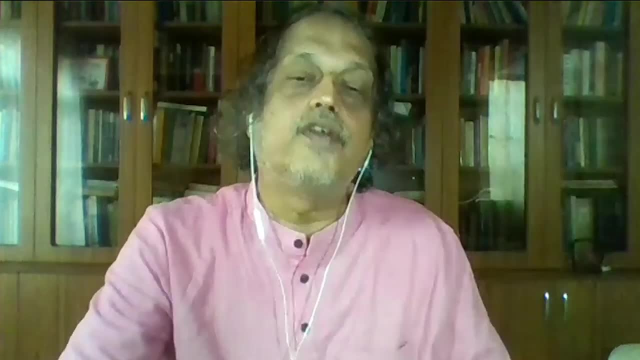 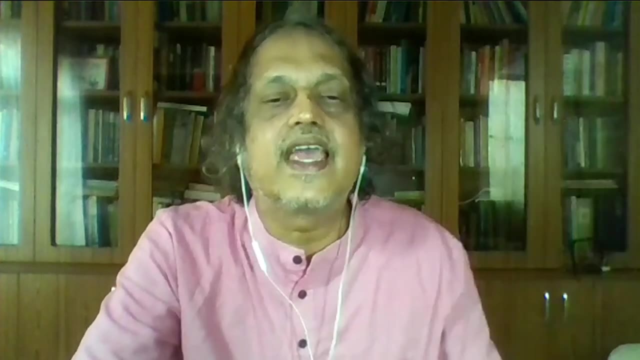 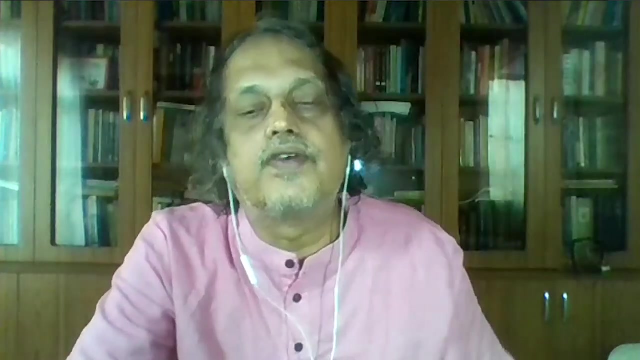 concepts that philosophers have written about. do we talk about philosophers? do we drop all the names of famous philosophers? if so, which ones? since the philosophy books are heavily biased against and ignorant about world philosophies, they are completely captured by a few philosophers in the name of philosophy. so first, and this was another very important lesson in this attempt to teach, 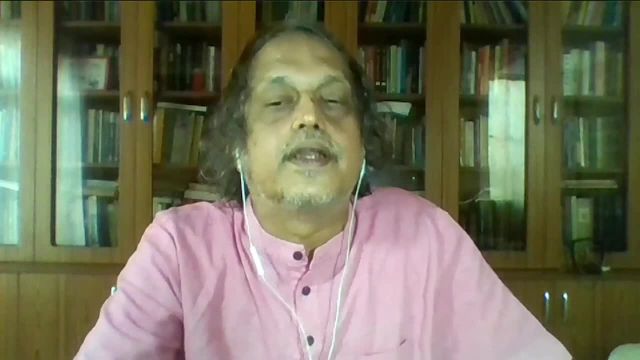 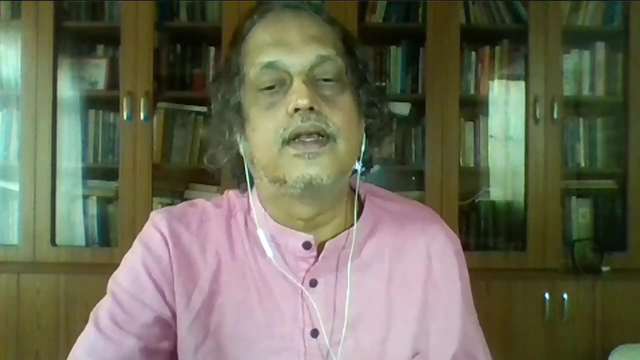 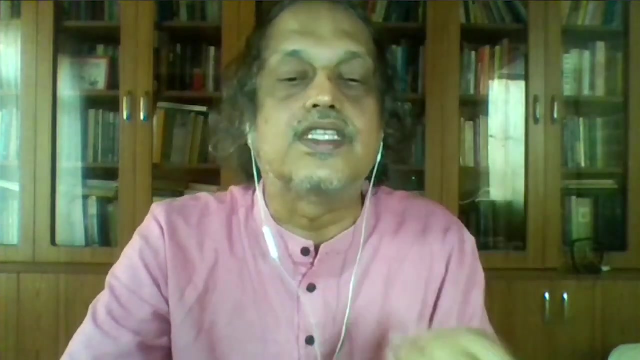 philosophy to children. firstly, I realized that philosophy to children had to be taught in a foundational manner. just like mathematics is taught as a foundation for learning the sciences, they don't teach mathematics by starting with what a mathematician said or how he or she presented a particular concept. the strength of mathematics teaching, particularly in schools, if 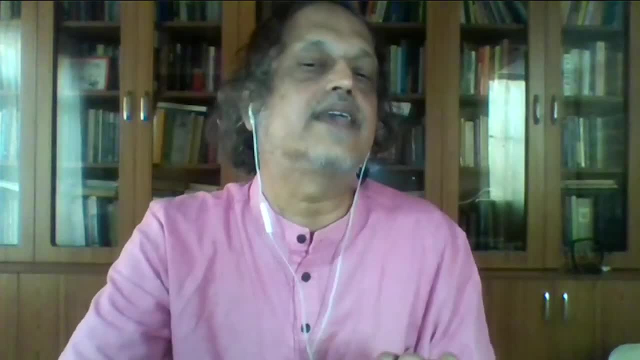 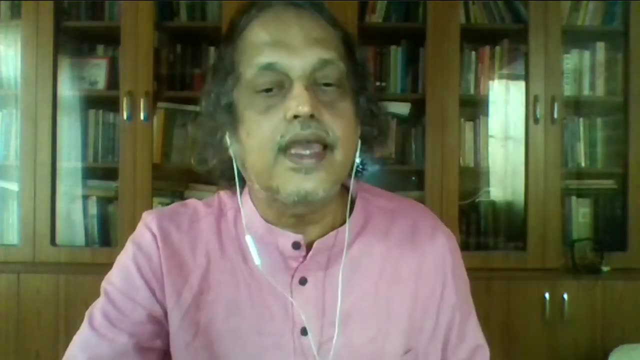 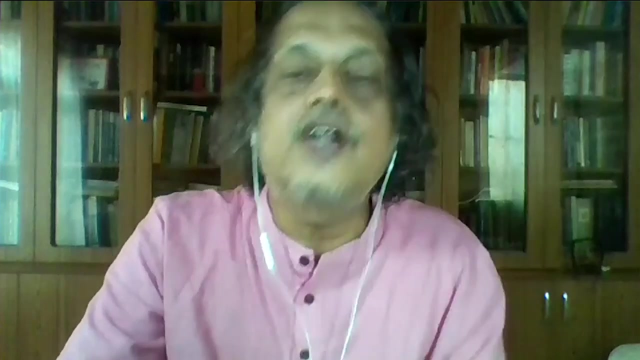 not at the higher levels- is on focusing on critically understanding and exploring concepts. secondly, I also realized that it was very useful to teach philosophical thinking through self reflection and awareness, and this brings the question of experience of learning into the content of what you learn, which is the content of what you learn and the content of what you learn. 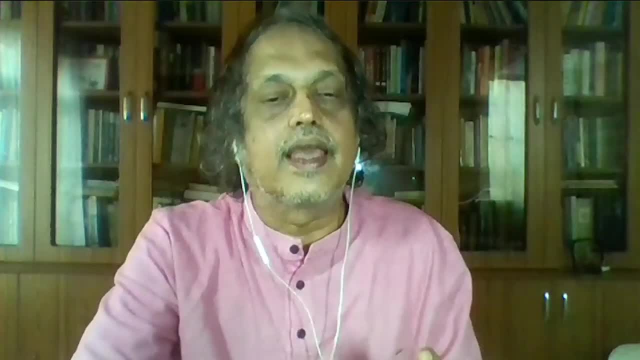 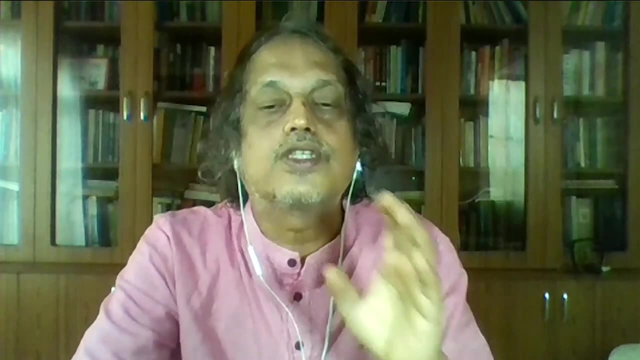 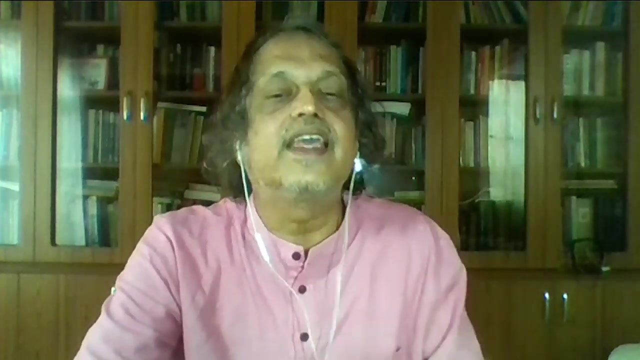 is normally not done in the sciences, for example. philosophical thinking became a way to become aware of our many cognitive and effectual processes. the focus was thus on making the students more mindful and aware of what they do when they learn something so much of core philosophical thinking. 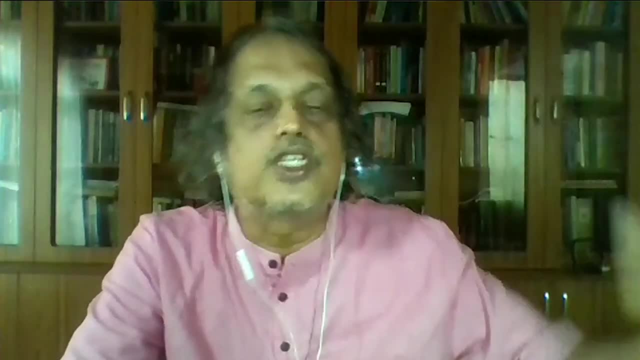 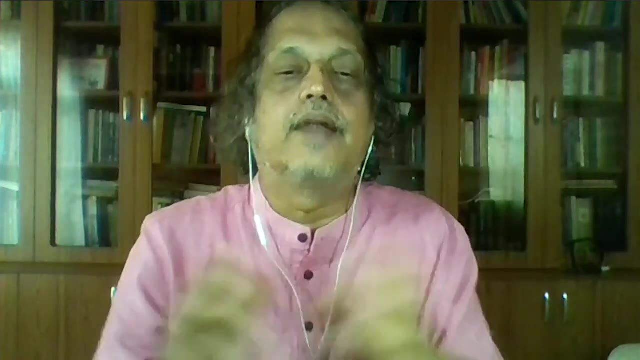 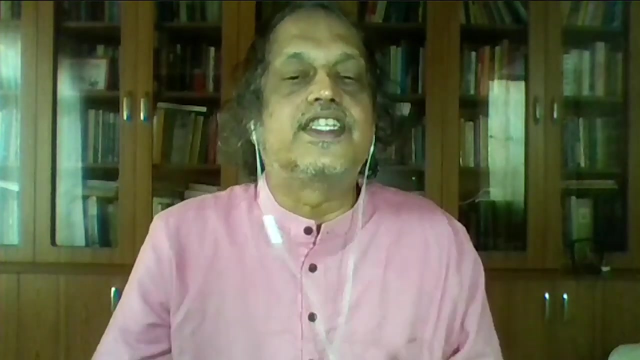 the basic ideas in philosophical thinking, like what is knowledge, what is truth, what is reality, etc. is present in the self-reflective acts, when you subject your experiences to questions and how you can explain them. what is real sense and what is real reality? and then you have to. 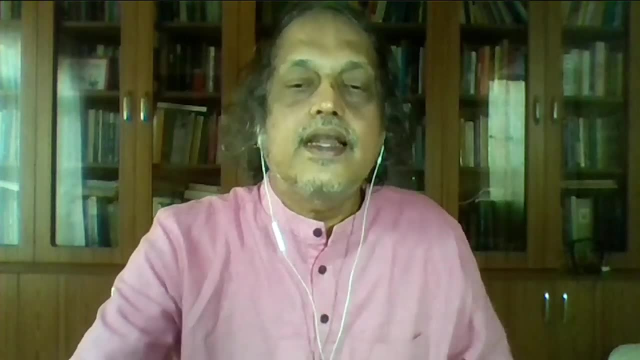 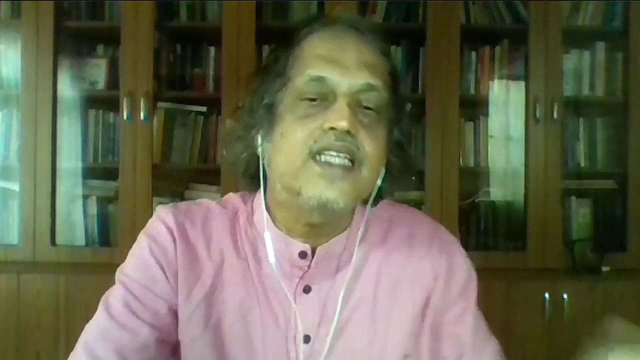 come up with a new opinion. and so now, why do I say that is sufficiently? we begin our workshops by thinking about perception and we ask the children to look at the chair, and ask them to look at the chair from different perspectives. then the children themselves start wondering. 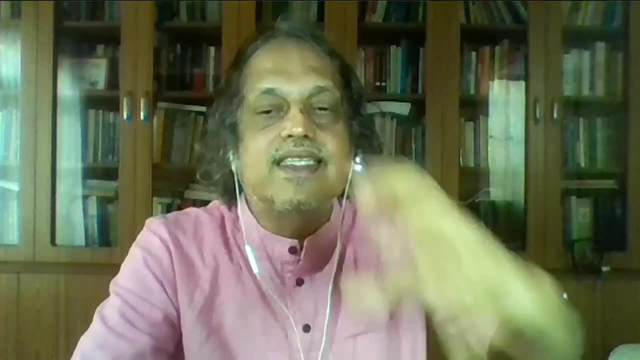 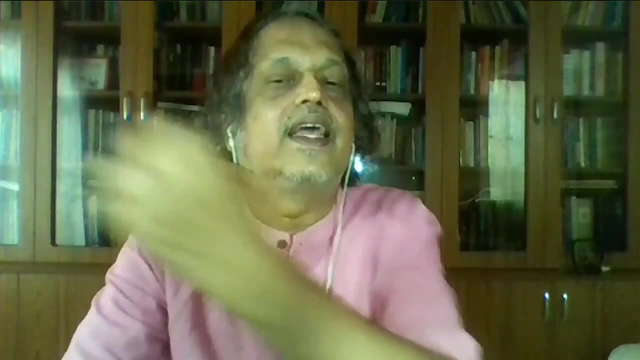 why, when each perception from different perspectives is so different, why is it that we call that say that object, the same chair? what gives that unity to these perceptions? are sitting in this workshop. What was that? Does something remain the same in oneself from the time? 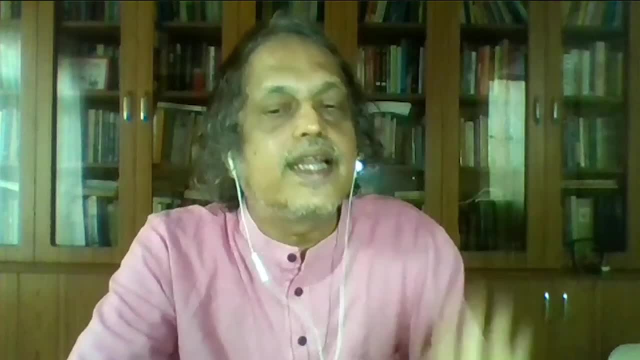 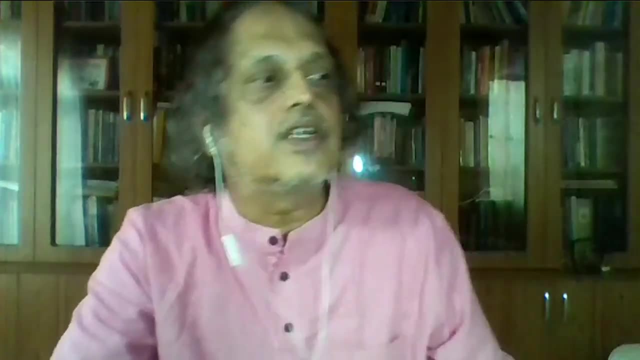 you're born to the time you are in now, And this also led them to think about similarities and differences. an important theme in philosophy, And the crucial point here is not just about talking about a perception of a chair and so on, But what we do with this is we extend it to the 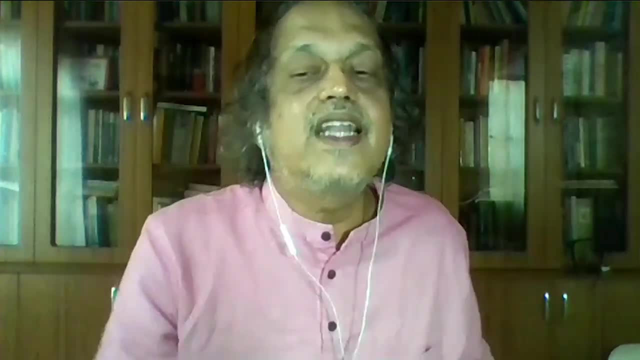 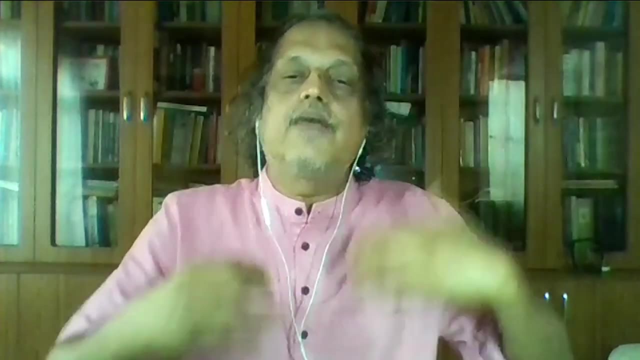 concepts and ideas they learn in their lessons. So this made them realize that, just as they could explore the different perceptions of the chair from different perspectives, they could do the same for ideas and concepts like numbers. What are numbers? How do you look at them from different? 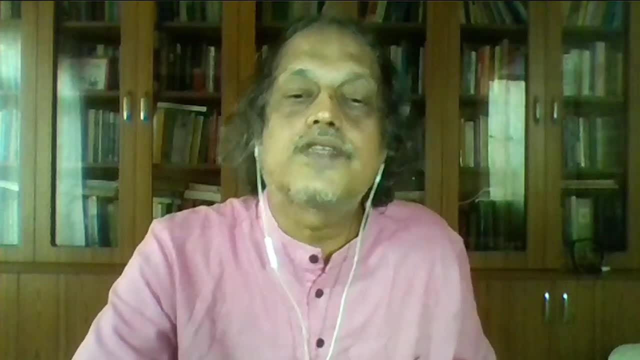 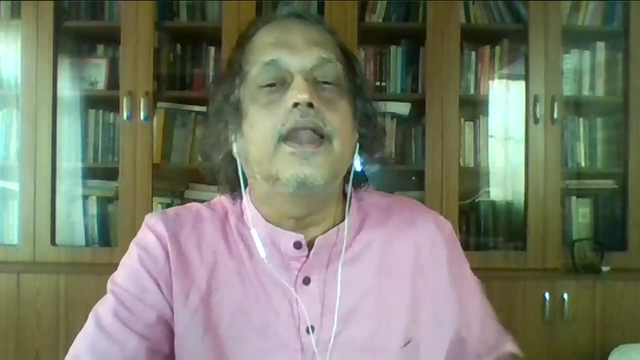 ways, Ideas of justice and freedom and so on. Philosophers will surely recognize some elements of the discipline of phenomenology in these kind of approaches that we tried. Now, from perception, it was a natural step to thinking, about thinking, which is also done through the process of self. 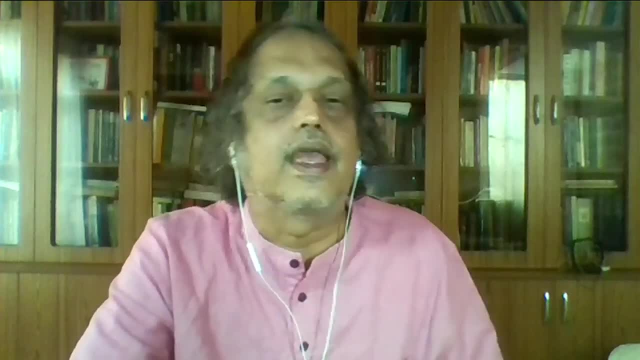 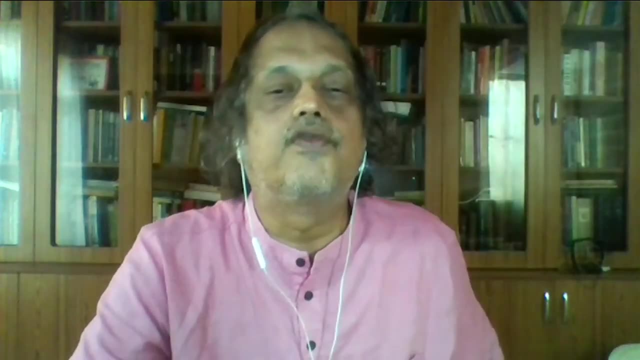 reflection. After all, there are experiences related to the process of self reflection. You know, every time you think there is an experience of thinking and we pay attention to that. So first we began by asking them to focus on the body processes related to thinking. 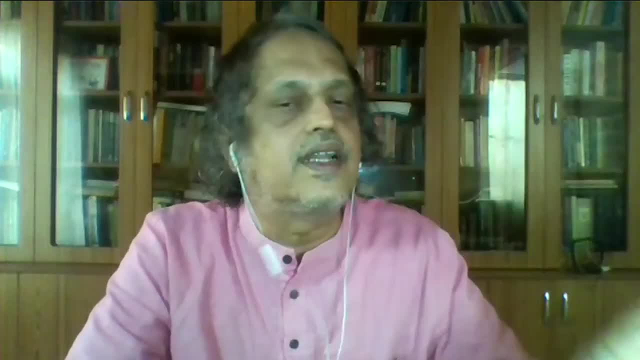 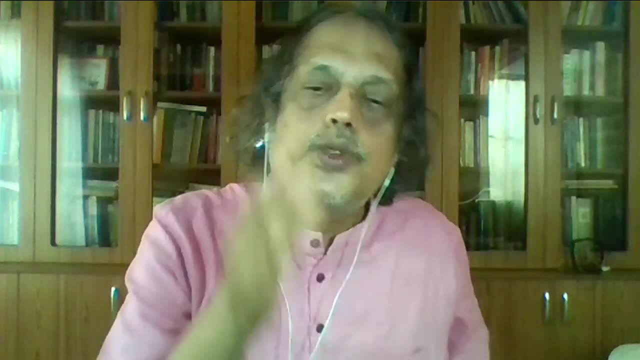 You know, whenever we ask people, are you thinking? all of them- all the children, like all adults, by the way- immediately say that they're always thinking. But the moment we ask them, what do you actually do when you think We got very interesting responses. Some kids said: 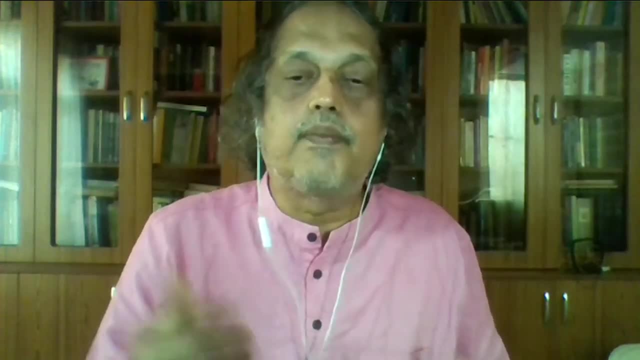 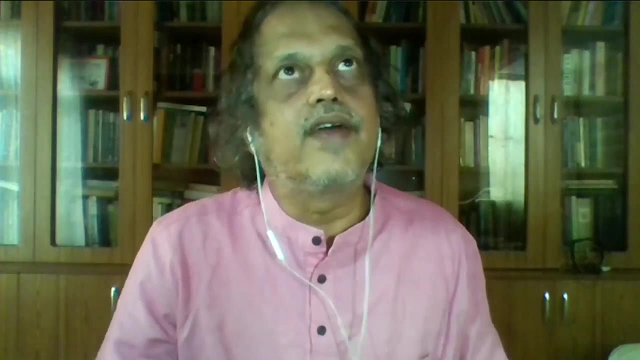 they get a headache when they think. So we asked them why they point to their heads whenever they say about thinking. And you know some kids actually it was very interesting. They thought a bit about that question. Why do they keep pointing to their head automatically when we 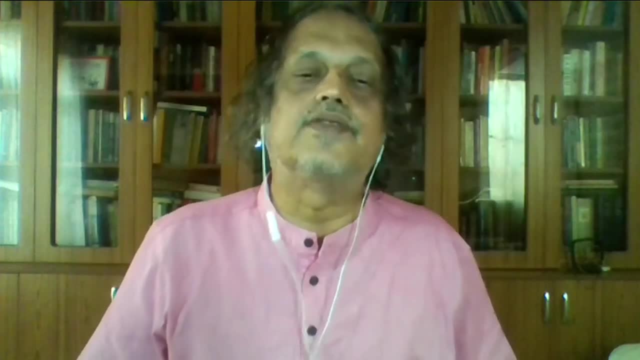 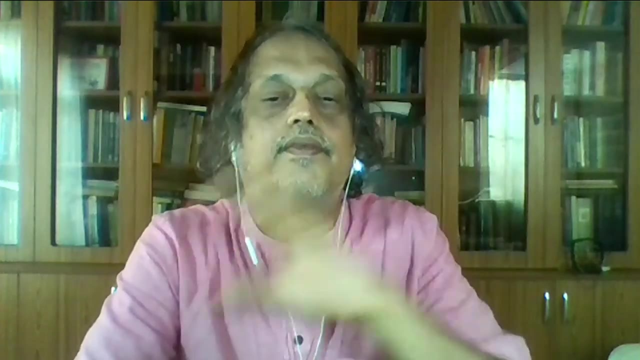 talk about think, And then some of them pointed to their tummies as a place where they felt thinking, And you know what is fascinating about this is they're correct, For after all, some of the very interesting theories of thinking also relate thinking to the gut And our most powerful. 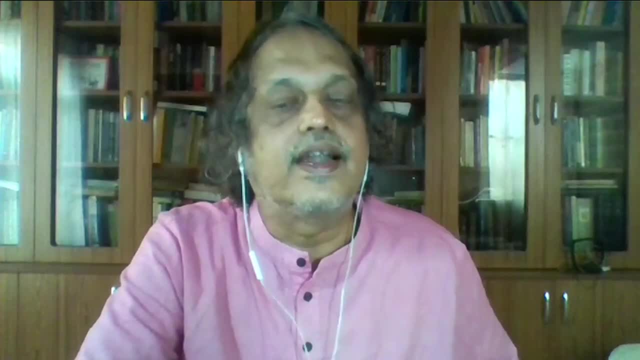 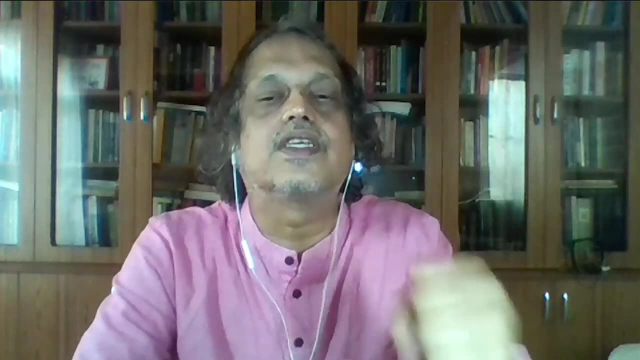 experiences of thinking and worrying, by the way, is actually felt in the gut. So you can already see from this how the children start thinking, not just by teaching them philosophical concepts and pushing the theories on them. to start thinking about their experiences of thinking, And they 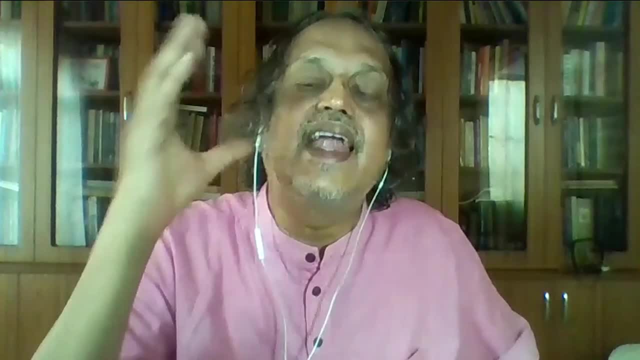 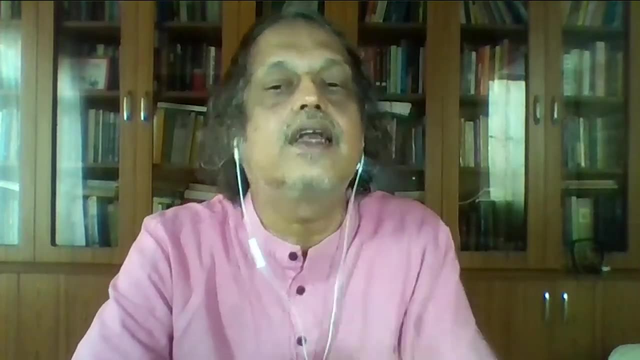 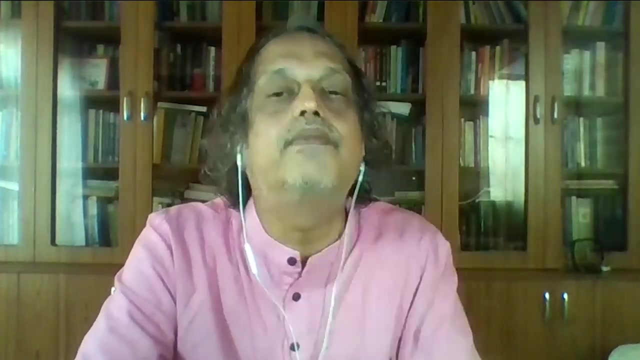 start thinking about the body doing the thinking, rather than blindly accepting the claim that it is the mind that thinks. So through this immersion to the experiences of thinking and raising many critical questions about their own experiences, the children actually stumbled upon some of the most important elements of the philosophy of body. 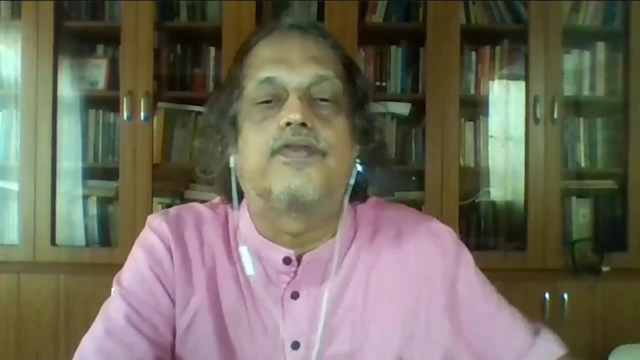 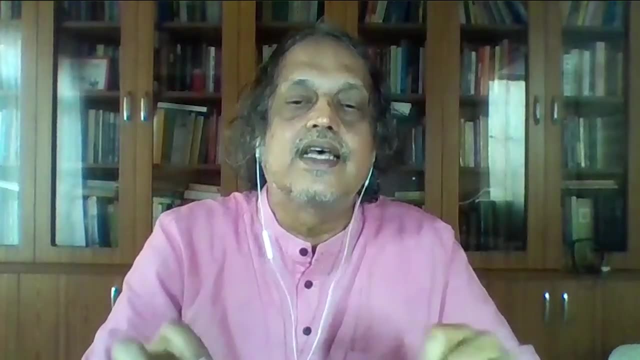 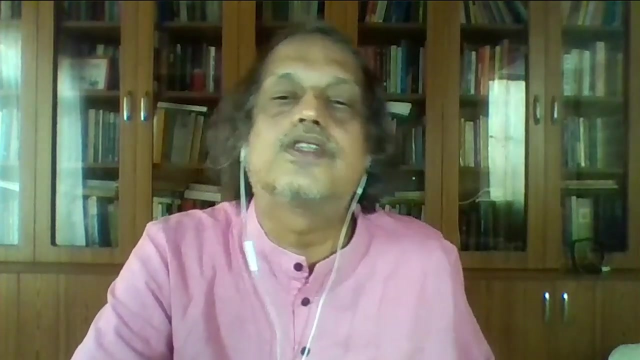 And mind. So rather than teaching them very complicated questions of philosophies of body and mind, there were kinds of conceptual grounding, conceptual grabbing of these ideas within children's mind as they learned philosophy in this manner. The second point about thinking that children responded to very strongly was the question of language in which they did the thinking. 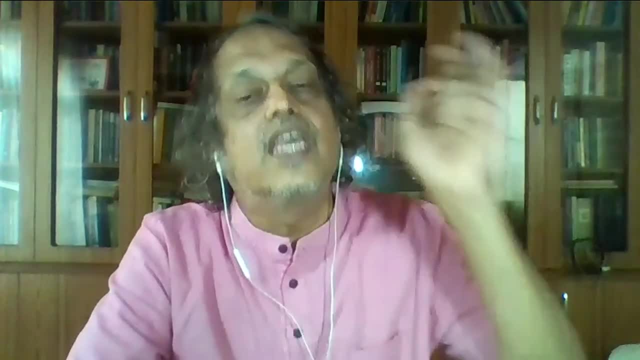 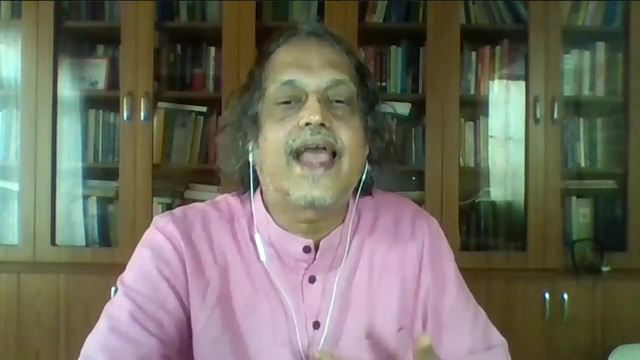 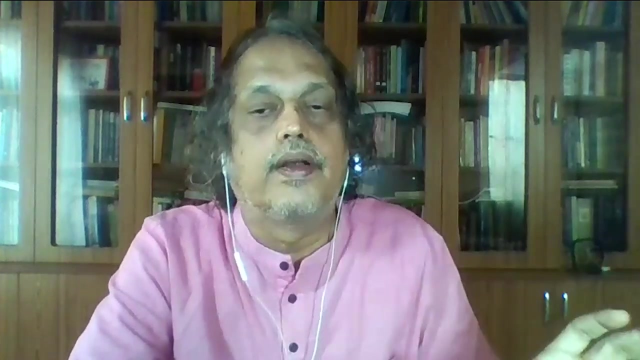 This issue is particularly important for a multilingual society like ours, even for science institutes like yours. Again, through your sections of questions and discussion, children learned how to communicate with language, whether they thought better in some languages, whether mathematical thinking was similar to thinking in languages, and so on. Now, one difficulty that we had in all this: 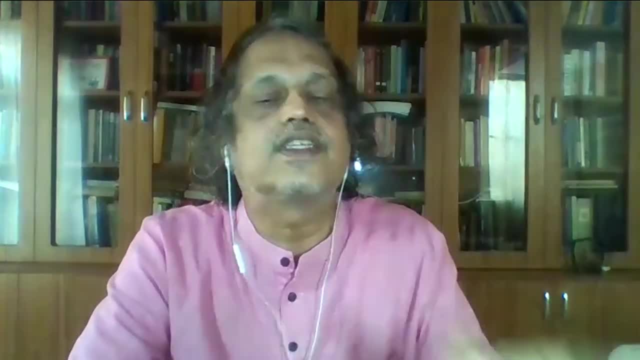 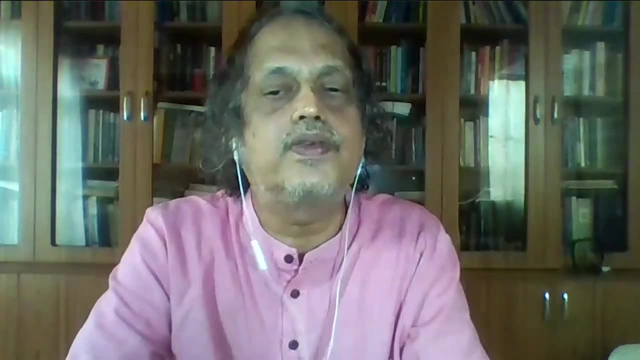 was that children had already been trained to believe that every question has to have one correct answer, And that's thanks to our great exam system. But the main strength of thinking is exactly the opposite, And we generally had some difficulty in convincing students to come up with multiple 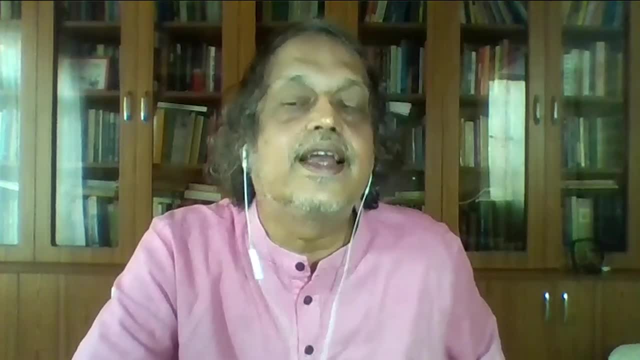 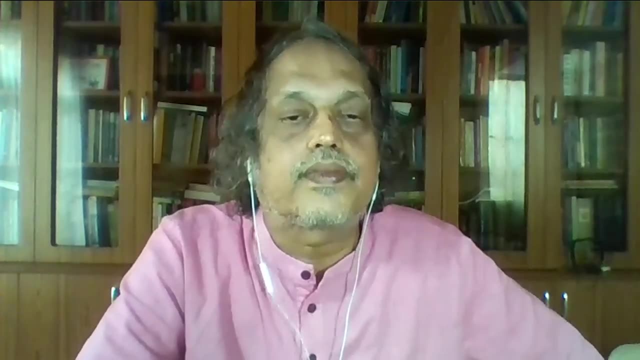 answers to a single question And when they actually realized that it was a single question- it is okay to say absurd answers to questions and produce multiple answers- they opened up quite effortlessly. We also found that the question of language liberates students enormously. 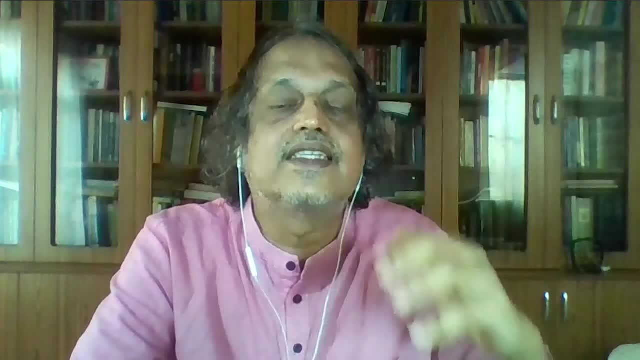 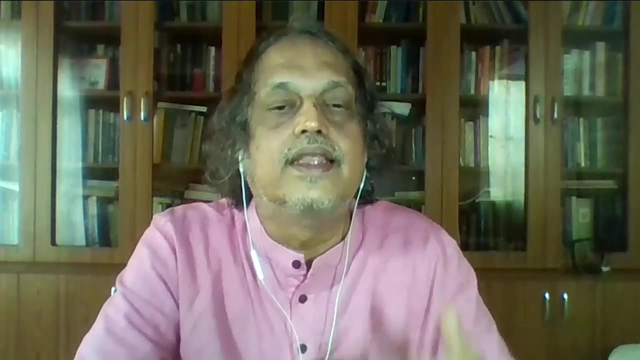 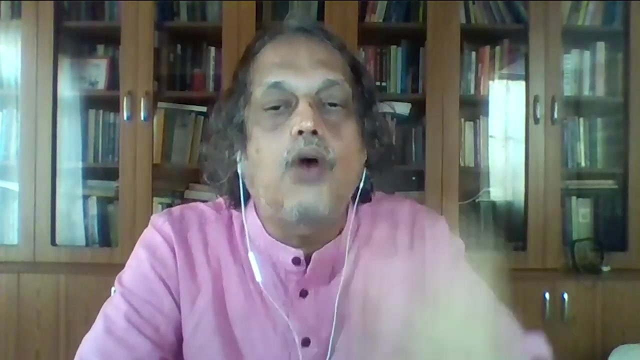 When they discuss the relation between language and thinking, they recognize that thinking is actually talking to themselves in some language. So it automatically led to questions of what language the children think in. They started understanding some of the basic questions in philosophy. They understood the basic principle of logic by analyzing how they come to. 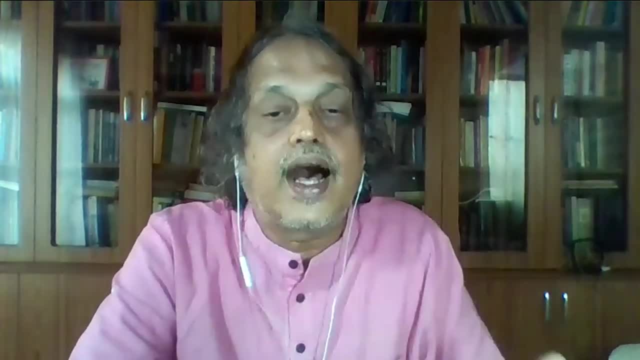 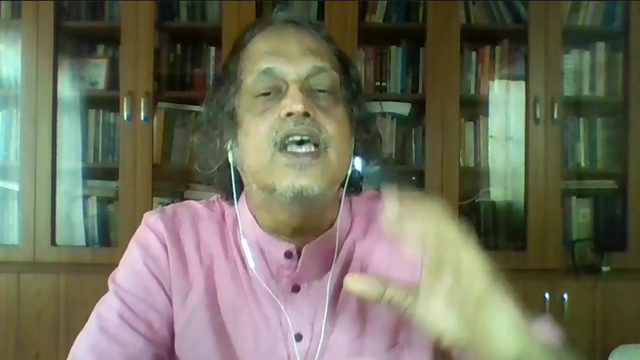 conclusions and how to use language to do that, And they also asked a very important question: whether strengthening language skills strengthen their thinking capacity. So what I'm trying to say is, once we start introducing the children to more and more deeper ideas, then actually they begin to. 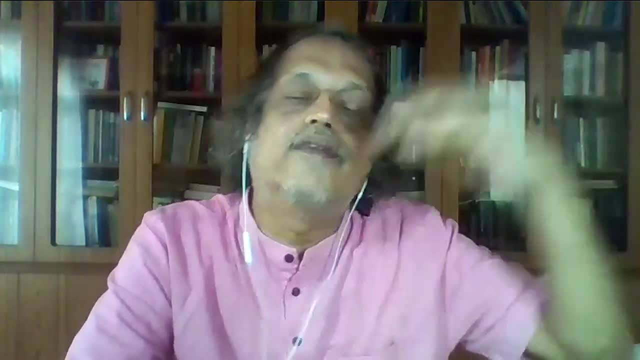 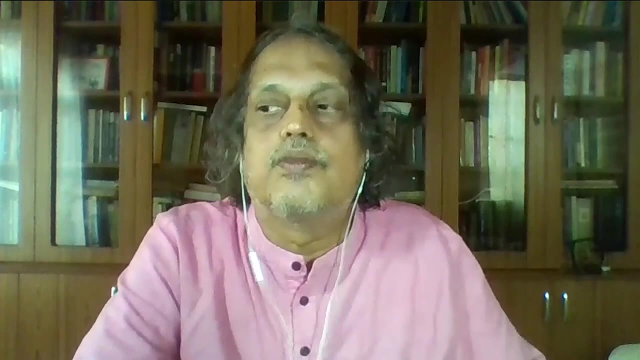 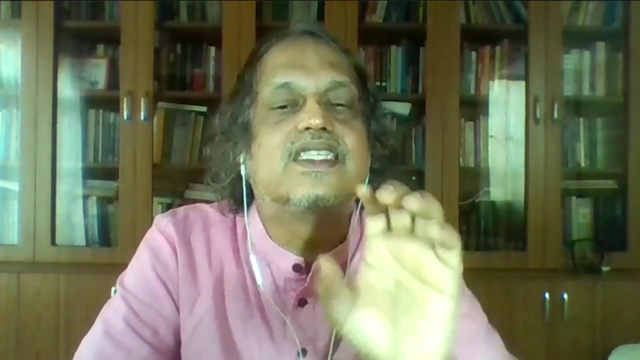 develop very rich ideas of what we would eventually call as philosophical. you know, philosophy in a larger sense. I have long argued that one of the most effective ways of teaching mathematics to is to use ideas of art and language And by talking about mathematical symbols and operations. 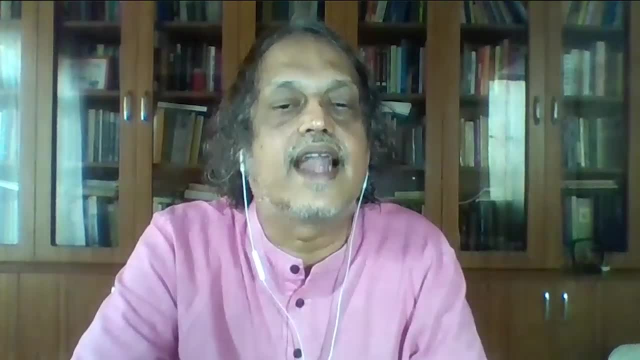 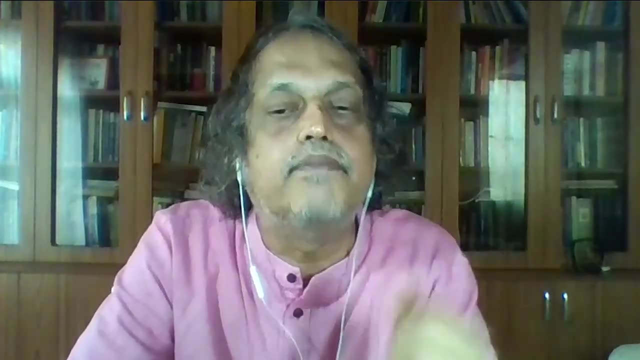 in terms of artistic creations and understanding them as we understand. language opened up mathematics to these students, So I'm not going to say they understood mathematics better, but when they start asking questions like what are numbers? Are they like other objects, Are they like characters? that 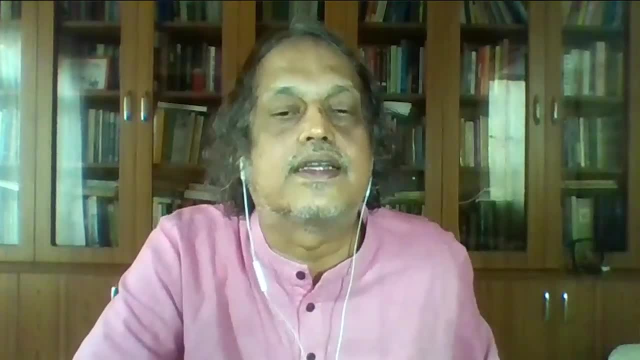 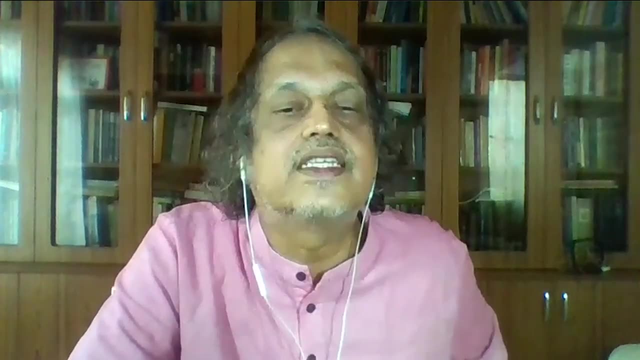 we see in comics? Do numbers have qualities, like chairs of qualities, etc. I found that many students derived great pleasure from recognizing that mathematical entities did not exist like physical objects. It actually made them think of mathematics as stories, narratives and as a 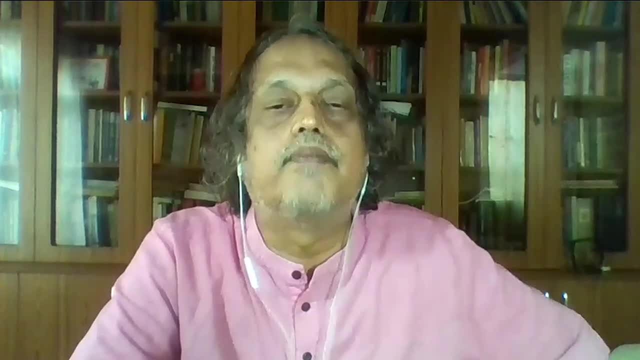 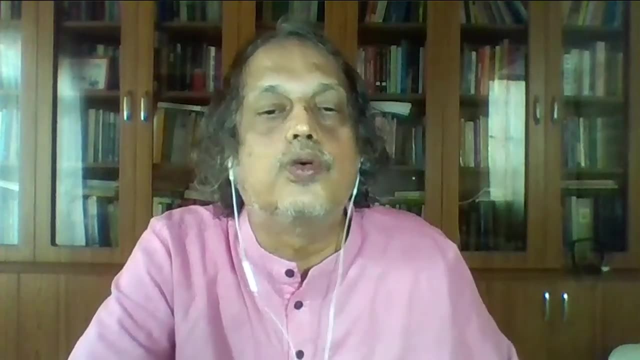 domain, which was very imaginative, And no session on philosophy is, of course, complete without ethics, And our experience was that it was the importance of teaching ethics through philosophy and not just as a list of do's and don'ts, Because there are moral. the states also have moral experiences.